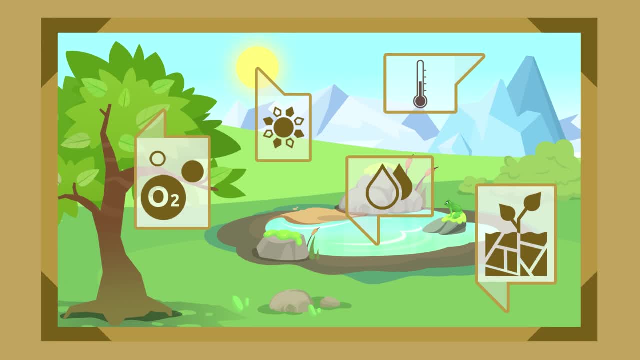 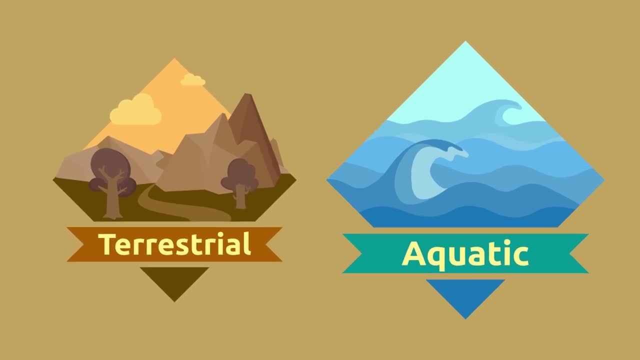 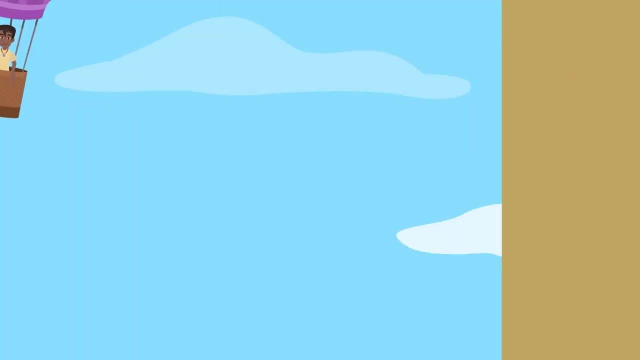 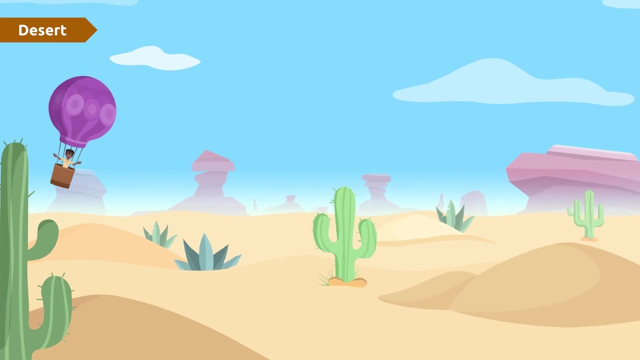 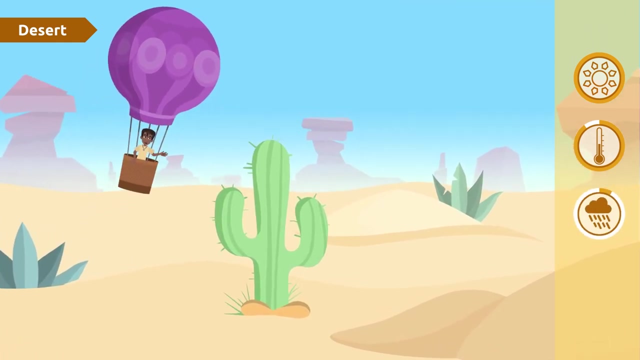 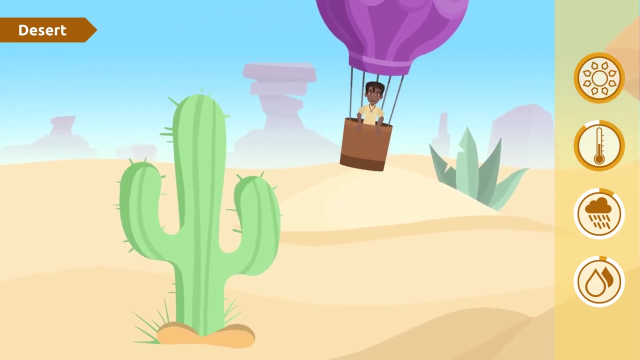 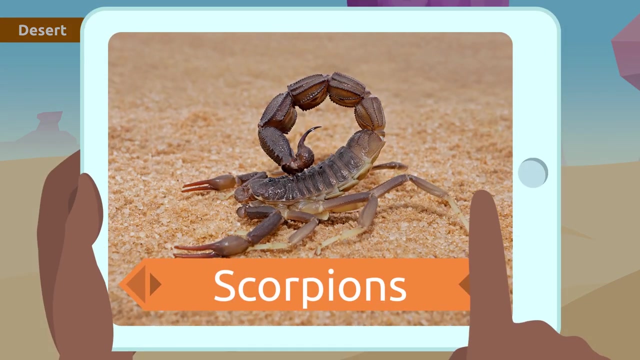 Depending on what these resources are, we can find very different habitats. There are two types of natural habitats: terrestrial and aquatic. Today I'm going to travel to the terrestrial habitats. Are you coming with me? Let's go. Snakes or mammals like camels or dromedaries can live in the desert. 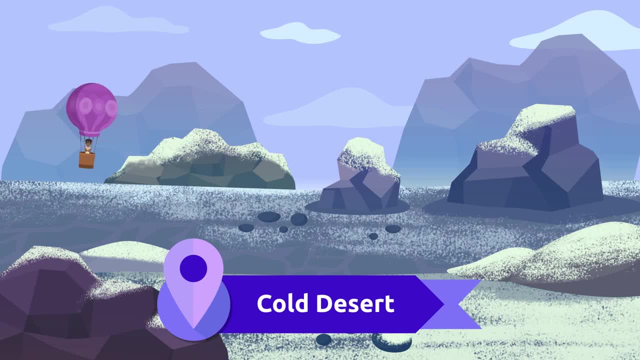 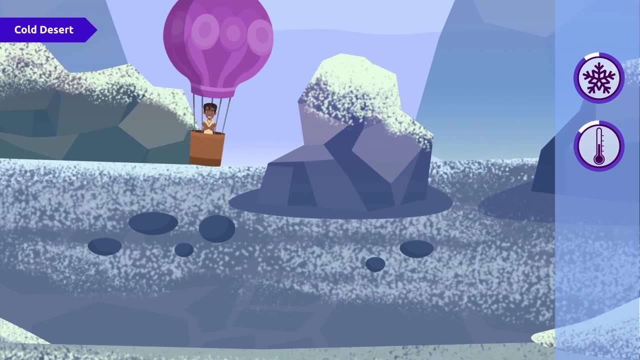 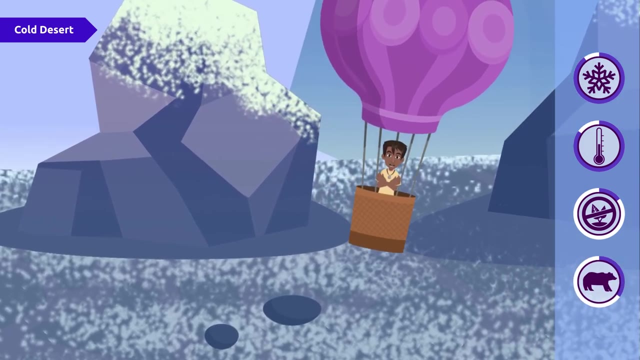 Did you know that there are cold deserts too? Here, everything is frozen and temperatures are extremely cold. There are barely any plants in these habitats. However, we are able to find some animals that have adapted to be able to live in them. 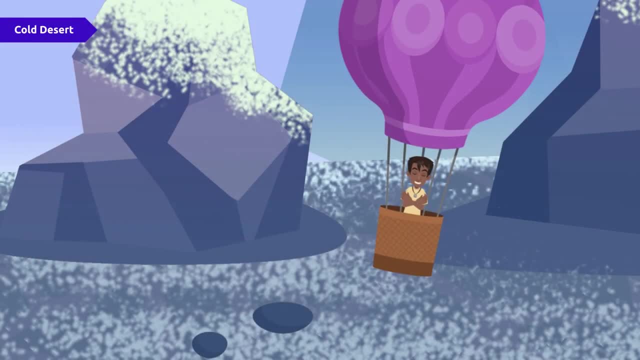 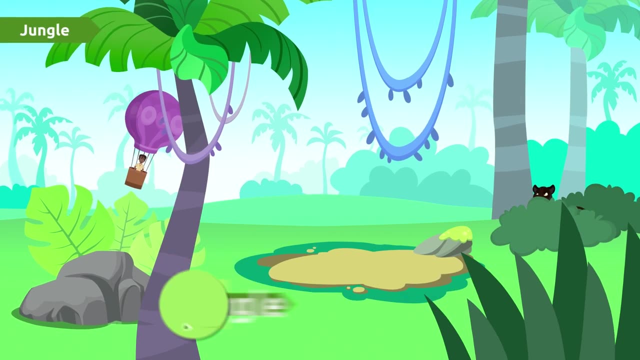 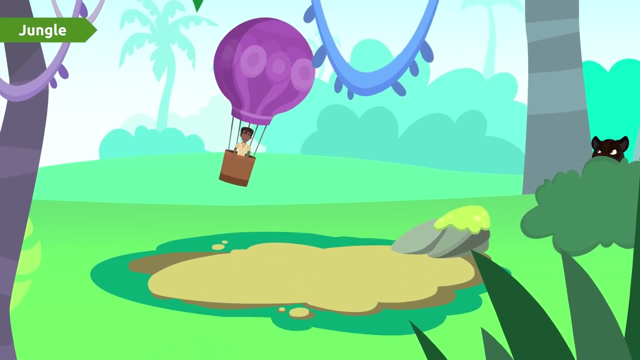 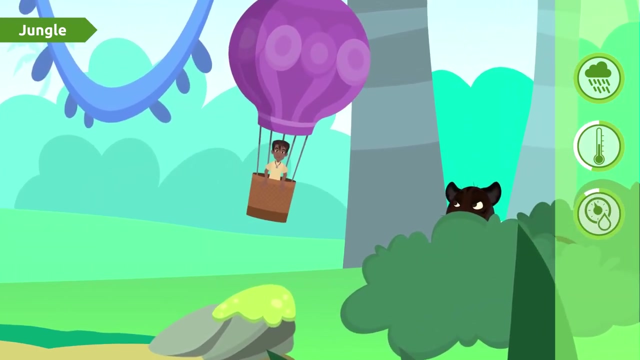 like the polar bear Jungle. We continue our trip. Look how many plants there are. This habitat is the jungle. Here there's lots of rain and temperatures are mild or warm. This favors a humid environment in which there are many living beings. 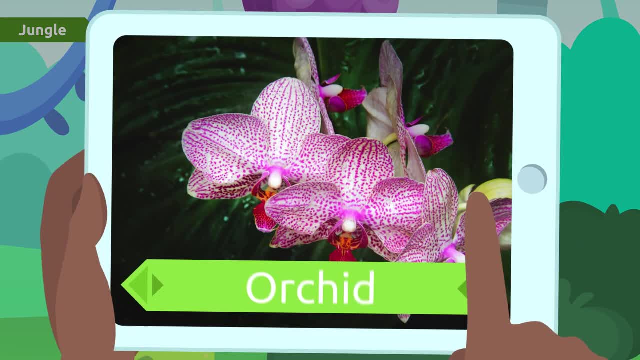 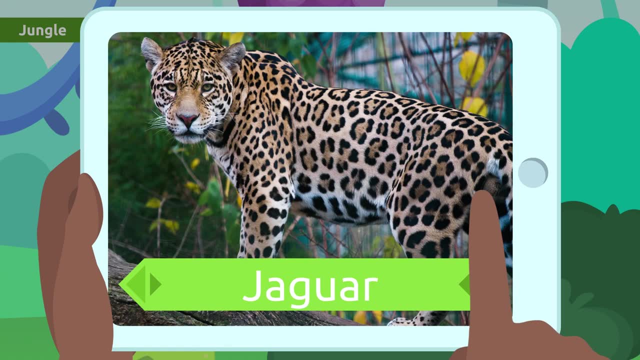 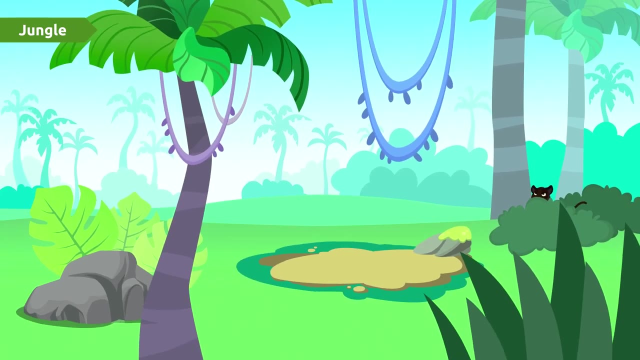 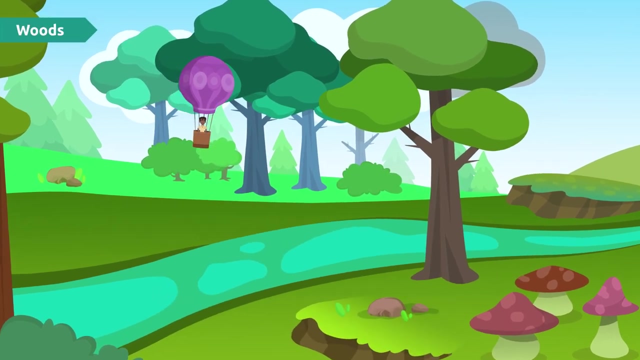 Let's see which ones we can find here. Look, an orchid And a hummingbird. This can be a panther or a jaguar. I think I'm leaving. I don't want to be his dinner Woods. We're in the woods. 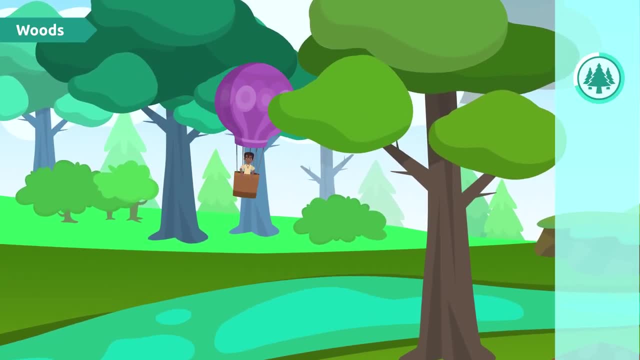 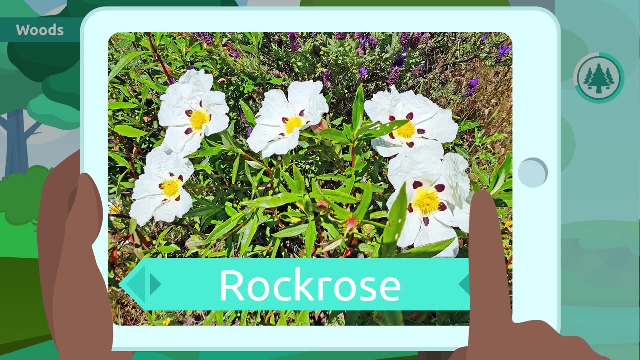 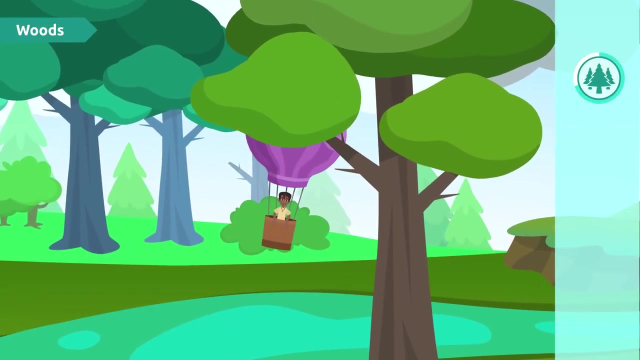 Here too there is plenty of vegetation, Mainly trees like beech trees or pine trees Or pine trees Or pine trees, And shrubs or bushes like the rock rose Or the arbutus. Did you know that there are many types of woodlands? 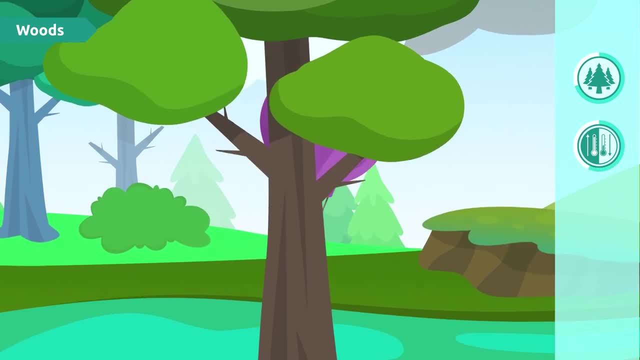 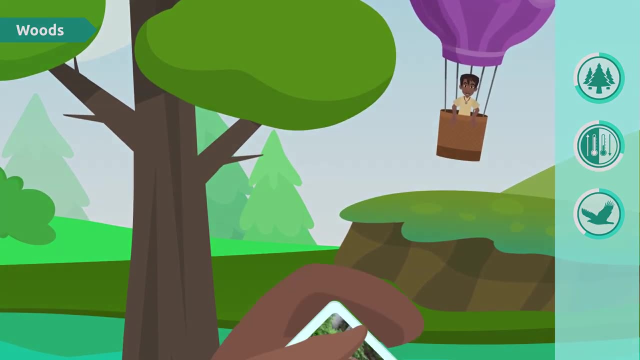 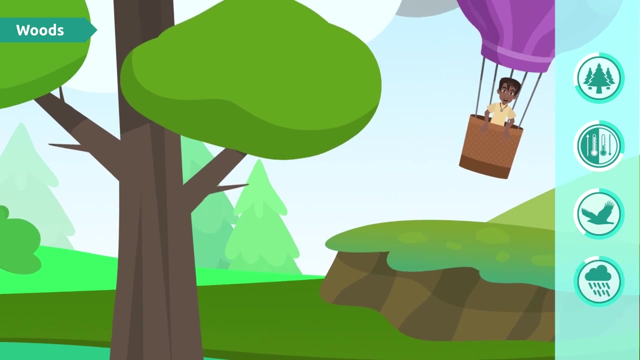 Their temperature may vary from cold to warm, And because of this the vegetation and the animals we find there change. In the woods, we can find some animals like bears or eagles. Here too, it rains often. I think that this cloud means a storm is coming. 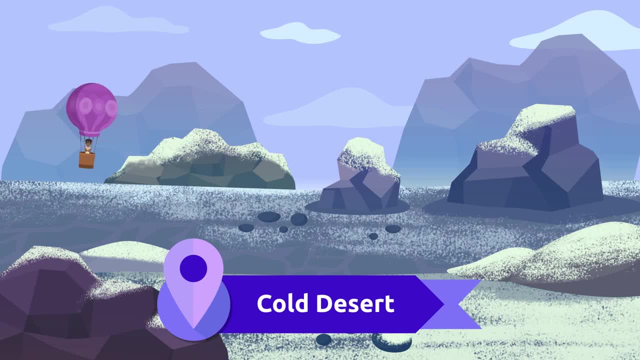 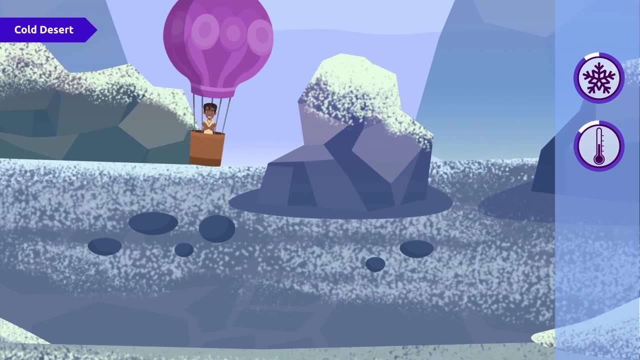 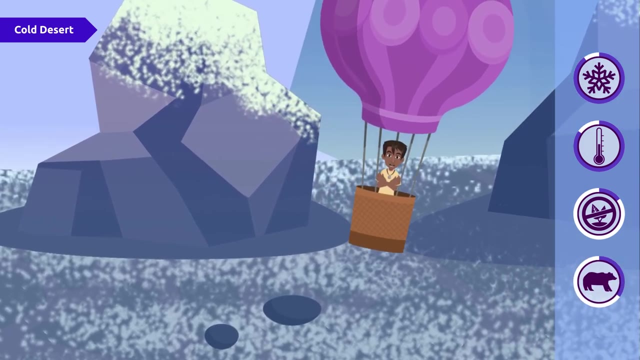 Did you know that there are cold deserts too? Here, everything is frozen and temperatures are extremely cold. There are barely any plants in these habitats. However, we are able to find some animals that have adapted to be able to live in them. 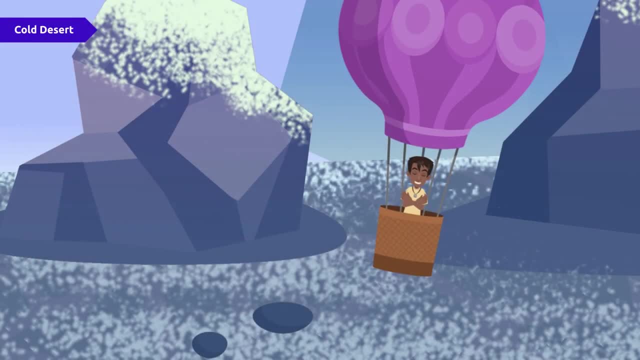 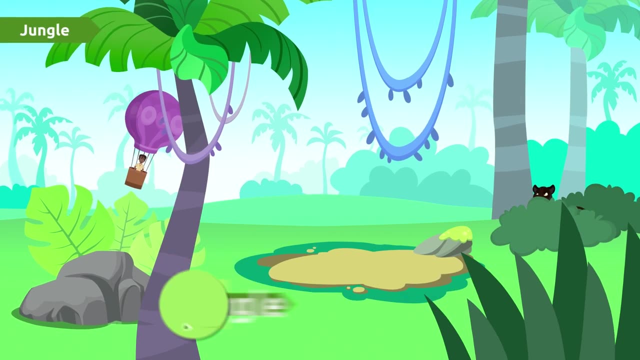 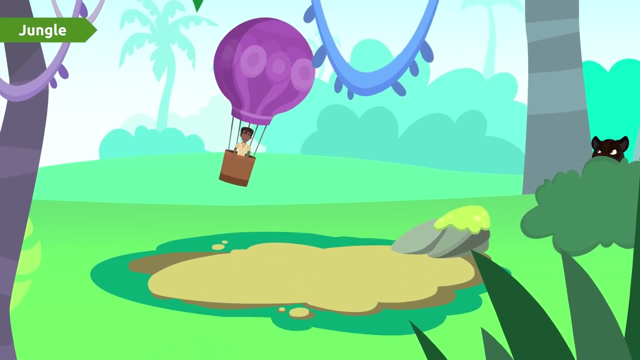 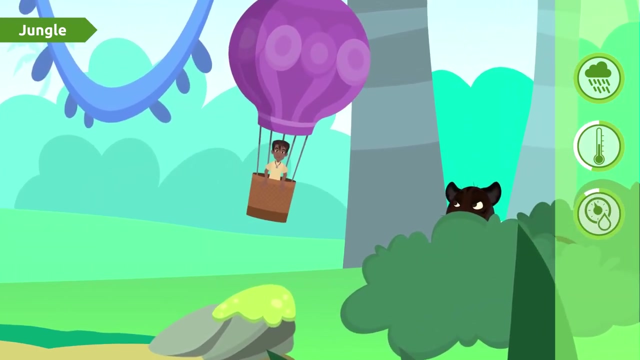 like the polar bear Jungle. We continue our trip. Look how many plants there are. This habitat is the jungle. Here there's lots of rain and temperatures are mild or warm. This favors a humid environment in which there are many living beings. 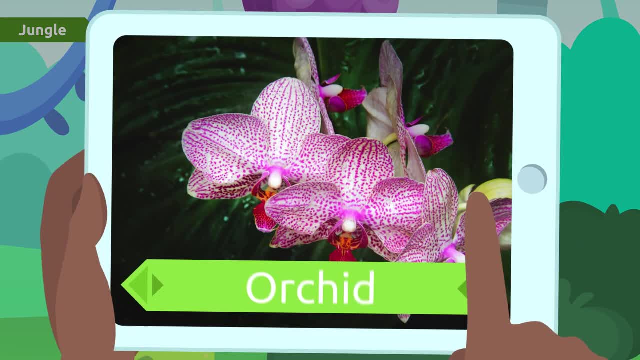 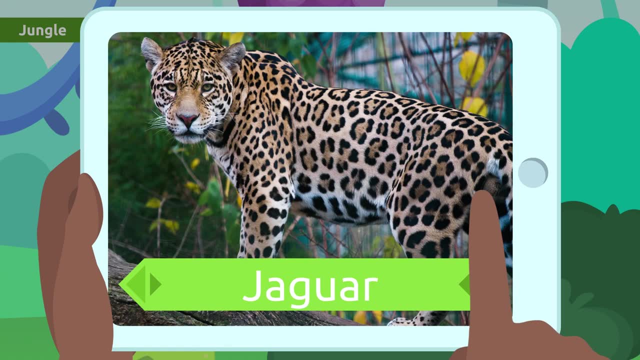 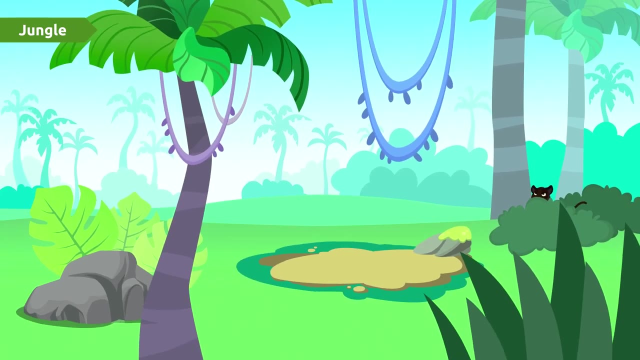 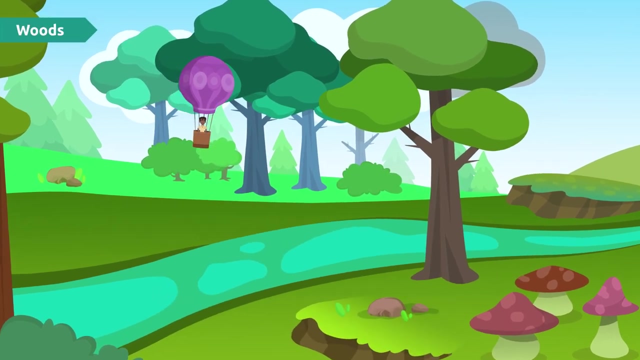 Let's see which ones we can find here. Look, an orchid And a hummingbird. This can be a panther or a jaguar. I think I'm leaving. I don't want to be his dinner Woods. We're in the woods. 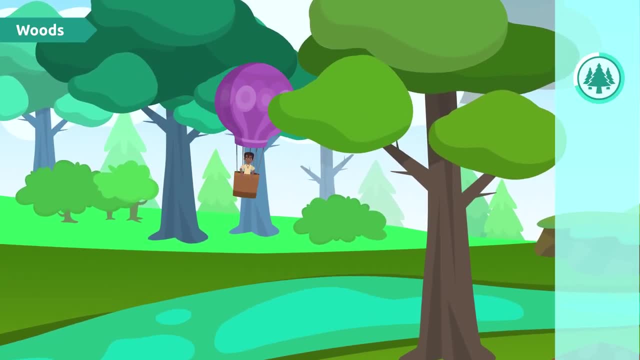 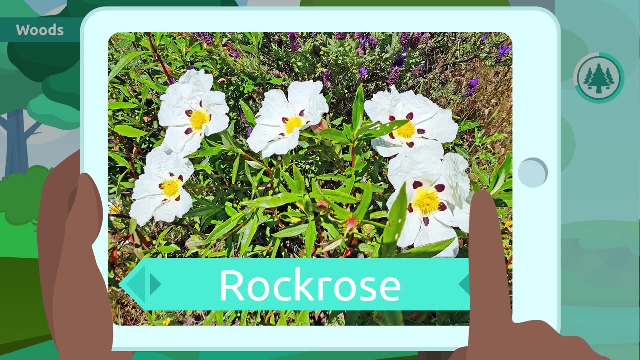 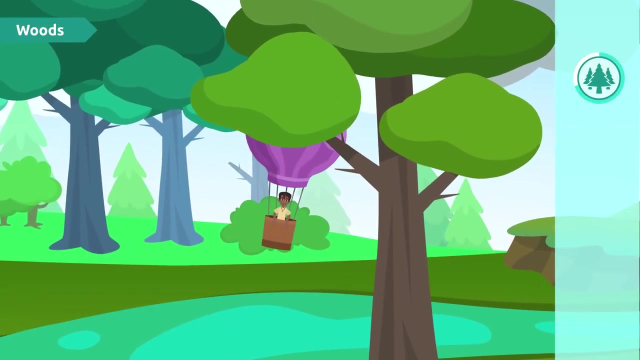 Here too there is plenty of vegetation, Mainly trees like beech trees or pine trees Or pine trees Or pine trees, And shrubs or bushes like the rock rose Or the arbutus. Did you know that there are many types of woodlands? 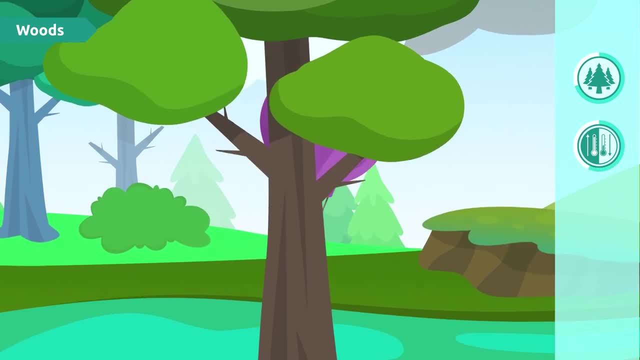 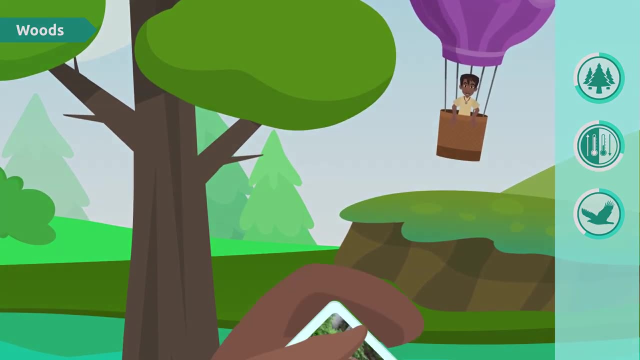 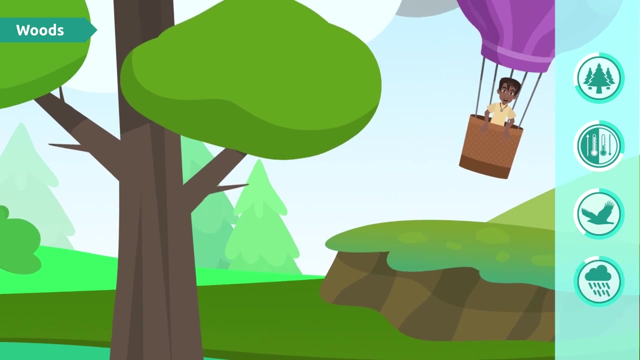 Their temperature may vary from cold to warm, And because of this the vegetation and the animals we find there change. In the woods, we can find some animals like bears or eagles. Here too, it rains often. I think that this cloud means a storm is coming. 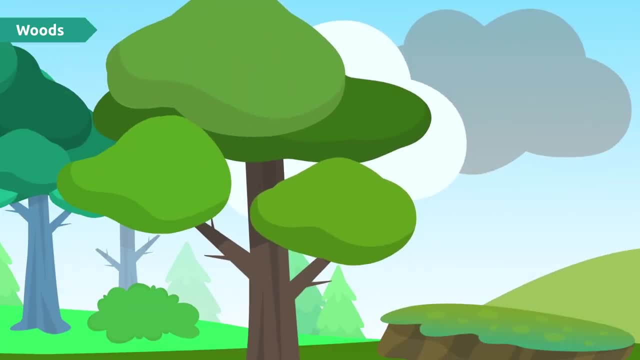 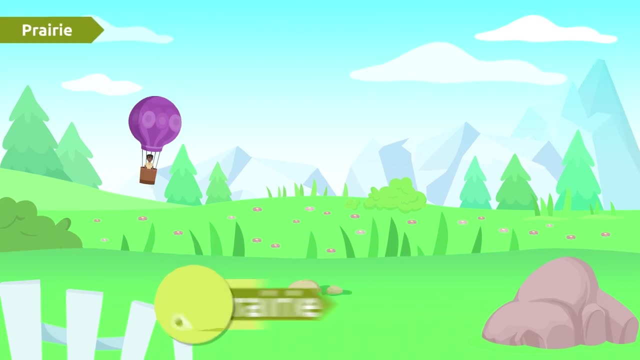 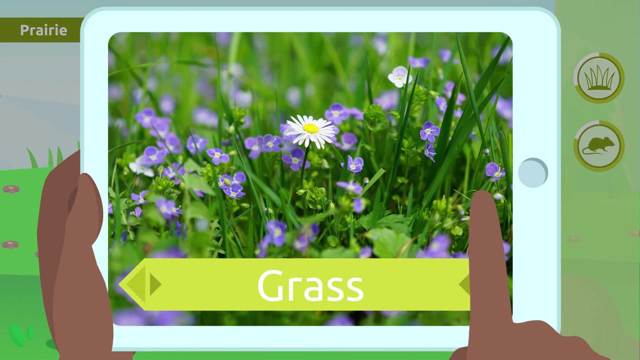 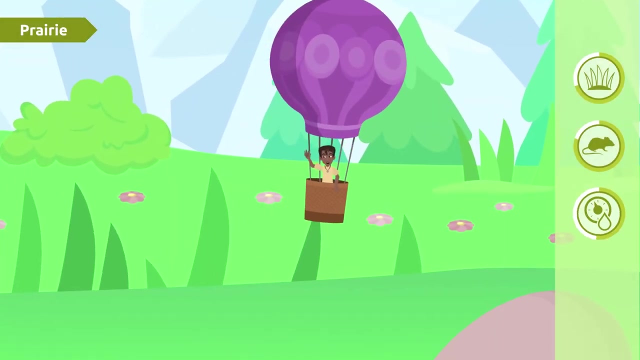 Let's continue our trip- Prairie. We've just arrived at a prairie. This habitat is characterized by small plants like grass, and animals like foxes or rodents. The climate in the prairie is humid, Winters are cold and summers are warm.